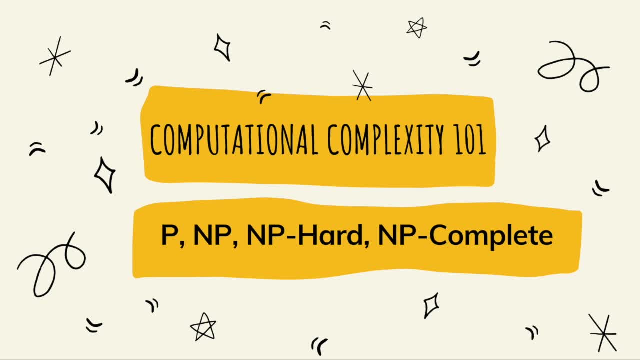 This is Computational Complexity 101.. If you've taken any algorithms class or anything related to do with problem solving, chances are that you would have come across many jargon terms like P, NP, NP-hard, NP-complete, and it's pretty common to actually ponder about what these classes or even 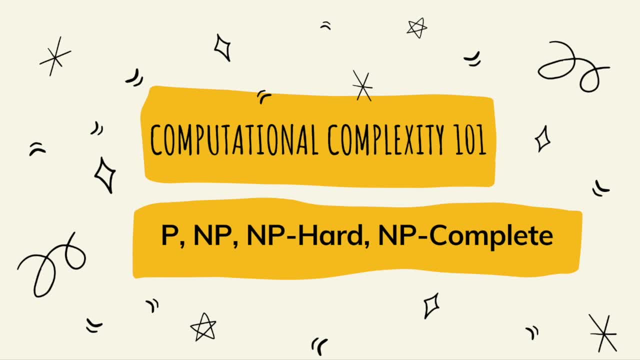 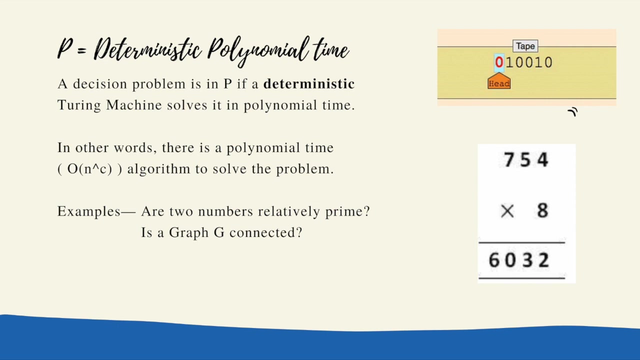 terms mean. So this is me making an attempt to simplify the computational complexity classes. that is thrown around at you, and let's get started. So what is P? I'll assume you have heard of something called Turing machine, even if you haven't, Just assume it's just a crazy machine, that with an infinite tape and it has like bits symbols. 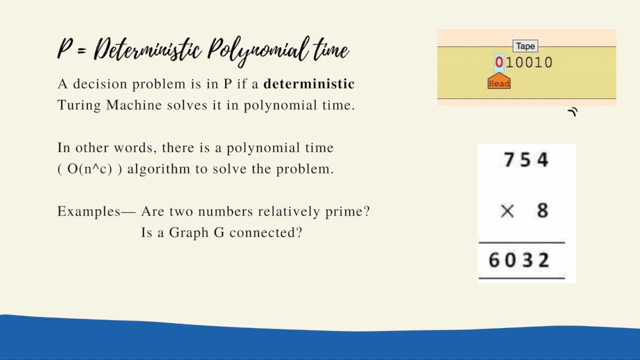 like zeros and ones written on it and it has something like a head and this, astonishingly, this crazy model, computational model that is proposed by Alan Turing is powerful enough to simulate any computationally known problem, So it's often used as a theoretical model to study computational complexity and many 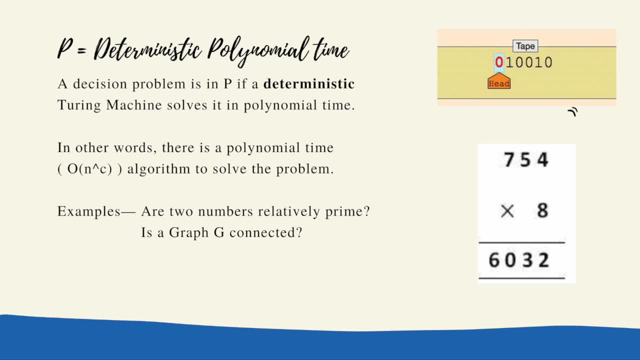 other things, and I'll often be using this Turing machine. It's just enough to actually know that this is a black box of some sort and it's okay to actually, you know, understand it as a black box for now, even if you have you don't. you don't know much about Turing machines, but 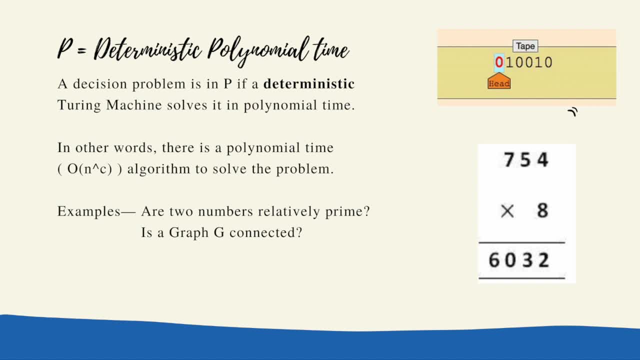 I'll relate Turing machines to computational complexity classes, and even if you don't understand them, you can obviously use them as a theoretical model to study computational complexity. You can obviously refer to a less toned down definition of the computation complexity and you will be fine. So let's get started. So what is P? P is a decision problem, and 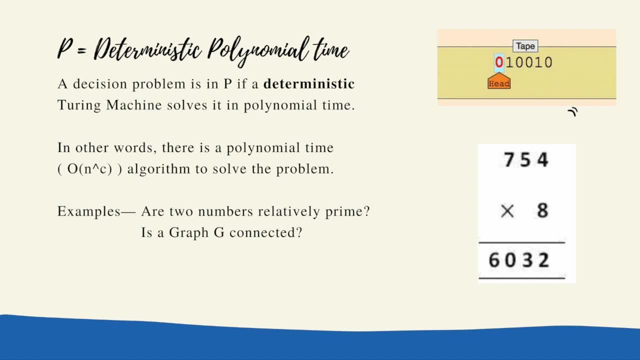 note what is a decision problem. Decision problem is a problem with a zero or a one or a yes or no answer to it, like, for example, is my given number a prime number, so it has a yes or no answer to it. And note that only decision problems are associated with these complexity classes, like P, N, P, etc. 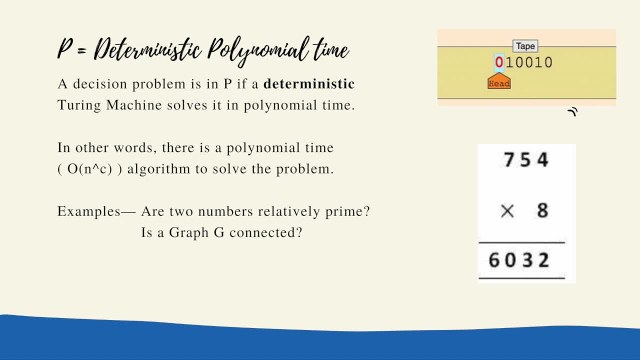 And there's also something called a search problem and that has a different complexity class associated with it. So generally, it's often a misconception to actually ask questions like: is an algorithm? like? I'll be talking about the conceptions in another slide, So let's just get started with this. So what is P? P is any decision. 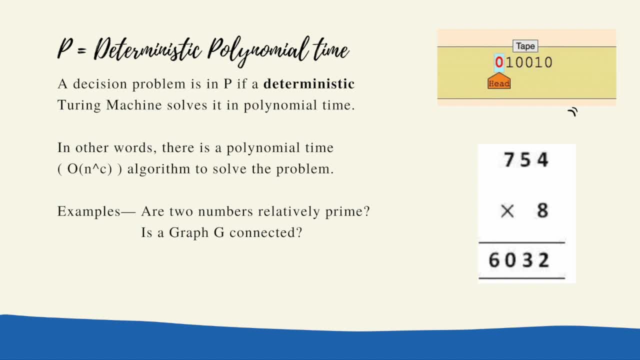 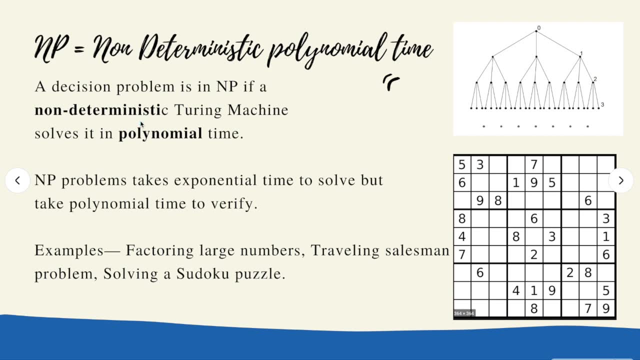 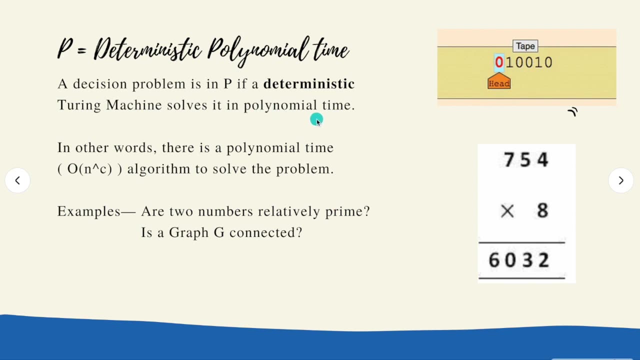 problem and that is solvable by a deterministic Turing machine. Deterministic Turing machine, Yeah, deterministic Turing machine in polynomial time. So I have polynomial time here and any deterministic Turing machine that's also in polynomial time, And in other words there is a polynomial time algorithm. Polynomial time algorithm is of the form N to the power C. That. 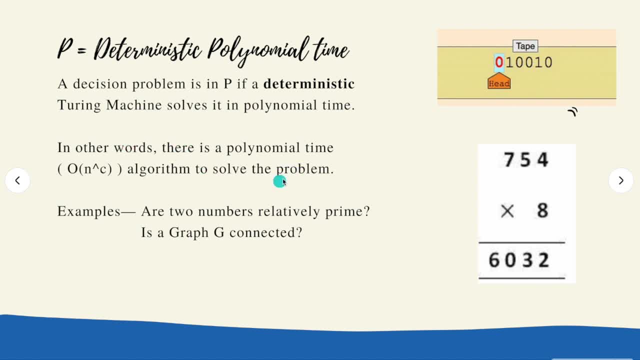 is known to solve the problem. So this is the definition that you should be fine with if you do not have an understanding of what a deterministic Turing machine is. So an example of that would be: are two numbers relatively prime? Note that two numbers are relatively prime if. 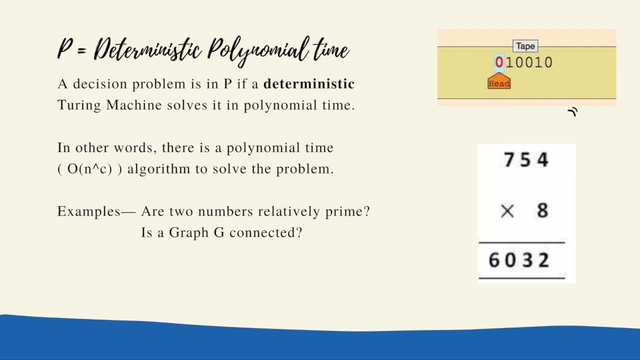 the DCD, the greatest common divisor of them is one. So an example of such numbers would be seven and five. They're relatively prime and you can obviously solve this in polynomial time. There is a good algorithm, called Euclidean algorithm, to calculate the GCD, And this problem is actually in P. Similarly is a graph G. 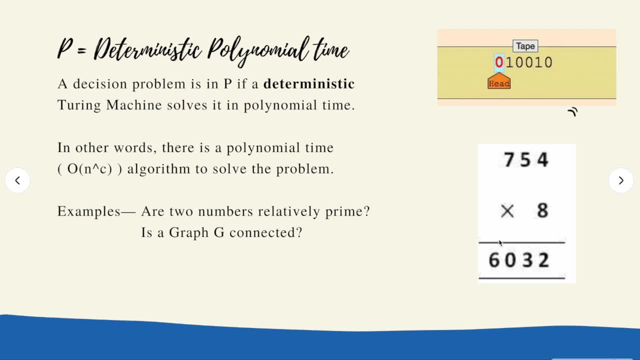 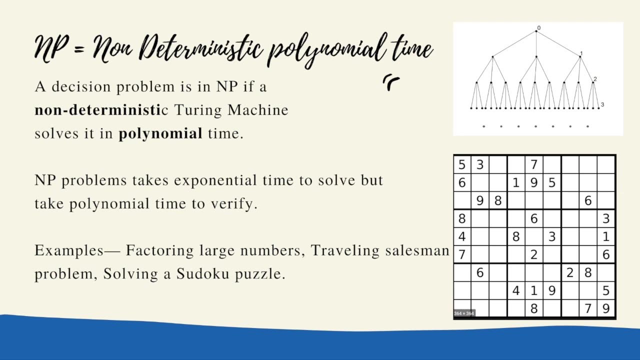 connected, That is, can I reach from any vertex of the graph to another vertex of the graph, And that's known as the connectivity problem, and that is also in P. So what is NP? It's a very common misconception that NP is not polynomial, And that is wrong. That is totally incorrect and in fact it's to do with 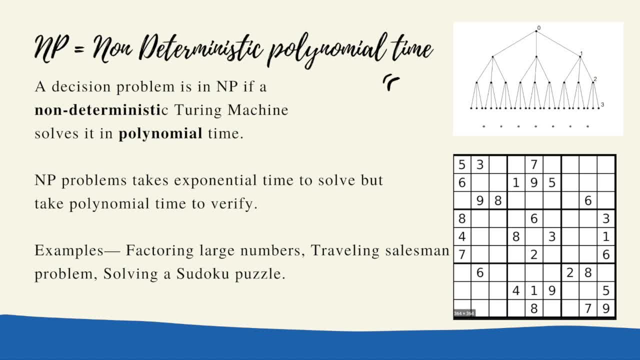 the notation and usually mathematicians or even computer scientists like in my opinion, they fumble a lot of notations And they make it very hard for people like us to understand anything to do with them. so it's not your fault, it's just to do. 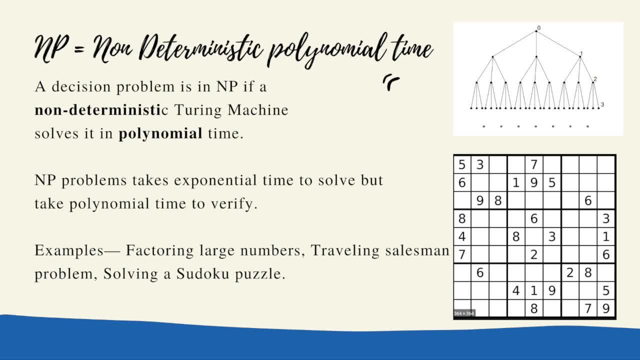 with the notation and NP is actually it is. it stands for non deterministic and not not polynomial. so in fact definition of NP is a decision problem. is an NP if a non deterministic Turing machine solves it in polynomial time. note, I'm using non deterministic Turing Machine here and a non deterministic Turing. 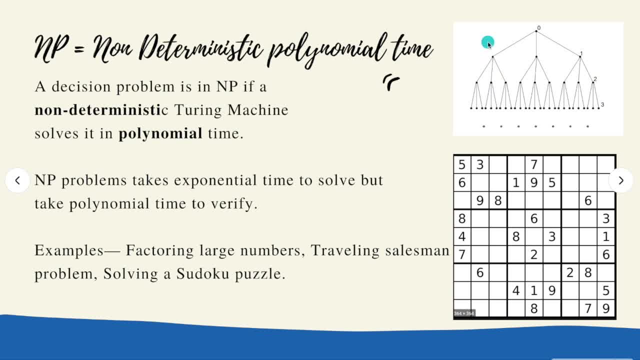 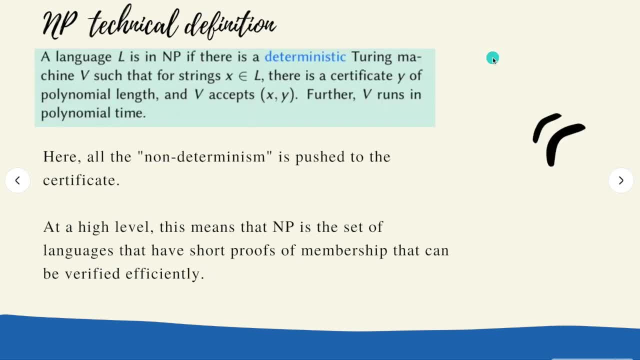 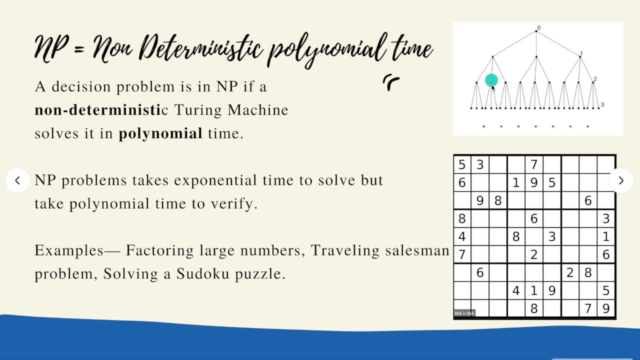 machine if you do not have an understanding. so anything to do with non determinism is like: just assume you here and you have to make a decision. you have to make a decision and if you pick choice 1, you're here, and if you pick choice 2, you're here, and if you pick choice 3, here. 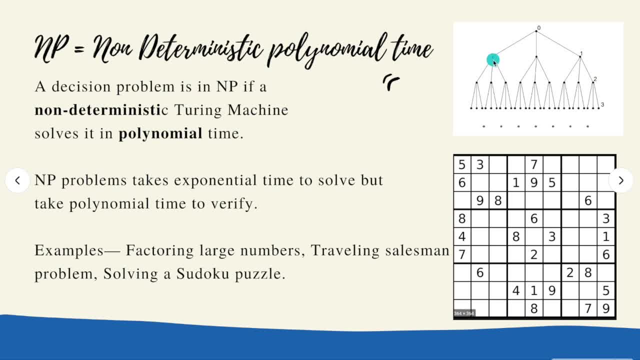 basically, you have ABS and assume that you're able to clone yourself three times at this particular point. this is not practical and this is impossible in real life, obviously, but non-determinism allows you to do that, and so, basically, the turing machine proceeds after having made all the choices, and it emulates all possible combinations. this kind of tree would. 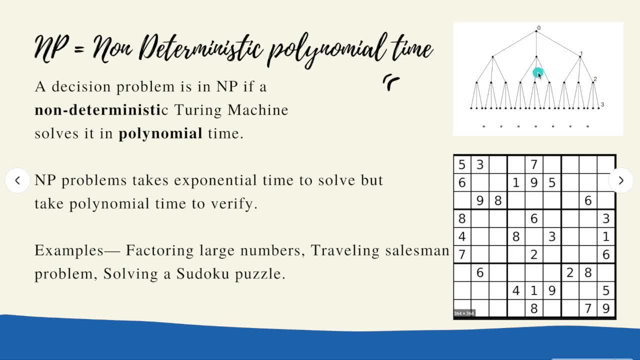 be very common in recursion problems. i mean, you've heard of it, but this is what non-determinism looks like: a turing machine is able to actually make multiple decisions at a particular point and is able to actually simulate all particular like possibilities and eventually, if there is any, 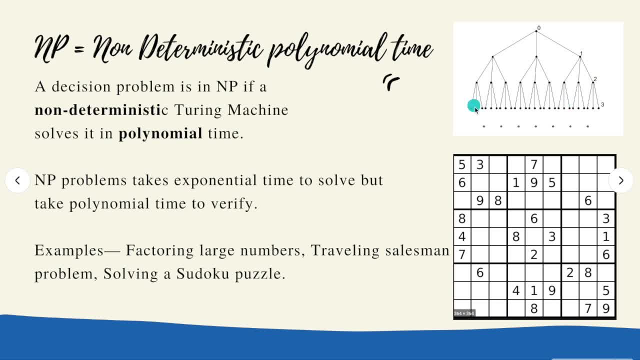 e s in any any one of the leaf nodes, the string or the problem is accepted or it's. the output of the problem is one that is, it's solvable or decidable. so that is non-determinism in a nutshell, not deterministic Turing machine in a nutshell. 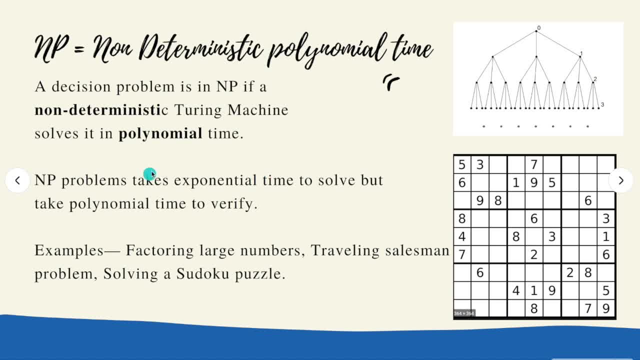 and if you do not understand that, and this has to be solved in polynomial time. so that is a definition of NP. know that it's polynomial and it's non-deterministic and it has nothing to do with not polynomial and, yeah, that is with the help of Turing machines and in. 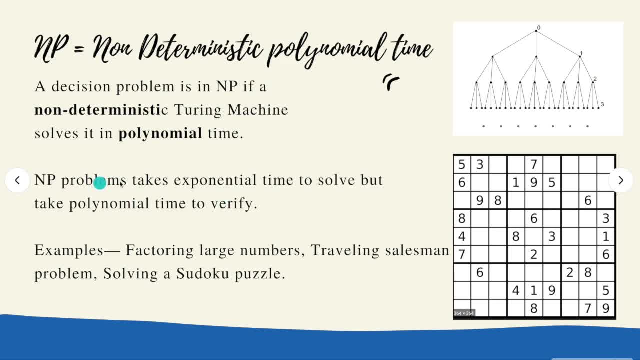 a nutshell. you define it something like this: NP problems take a very long time to solve. it is exponential, but these are the class of problems that are very easy to verify. and what does verify mean? to understand it easily, you can associate it. whatever I told you about NP to a 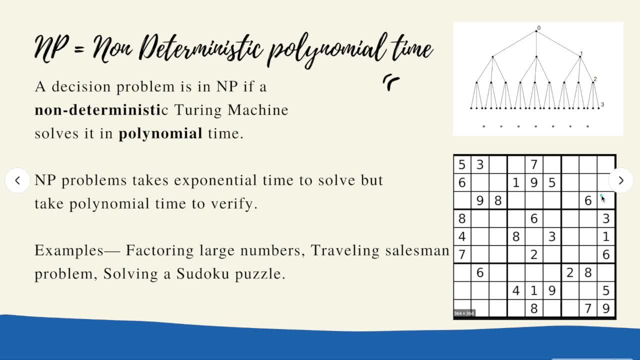 Sudoku puzzle and know that it's very hard to solve an n cross n Sudoku puzzle. normal Sudoku puzzles are 9 cross 9. that can be easy, but n cross n is definitely is actually a hard problem to solve. It's actually a difficult problem. it can take exponential time to solve. but hey, if I give you. 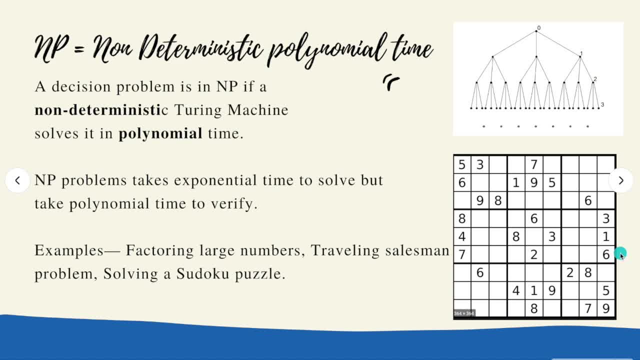 the solution to a Sudoku puzzle. it's fairly easy and takes polynomial time to verify that it is the solution of the given Sudoku board. so that is the definition of NP in a nutshell, and the examples of NP would be: factoring large numbers. yeah, note that this is often the basis of cryptography, like the fact that we cannot quickly factorize in. 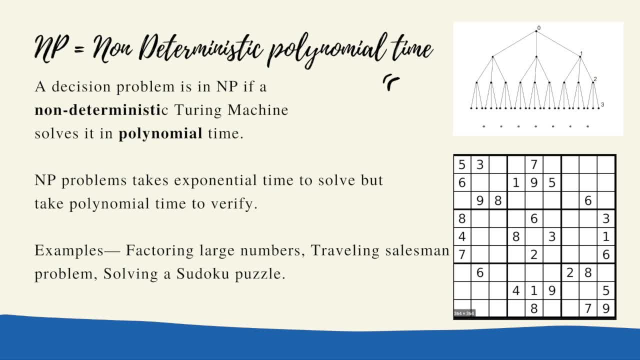 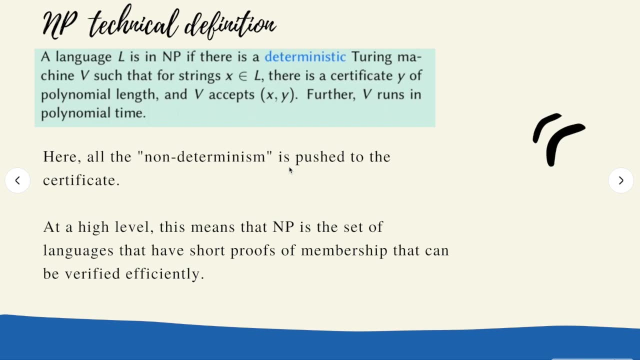 fact, like the prime, factorization of a very large number is often used as a building block to cryptographic algorithms, and we have the traveling salesman problem. and then solving a Sudoku puzzle is also known to be an NP. So, and this is the technical definition of NP, 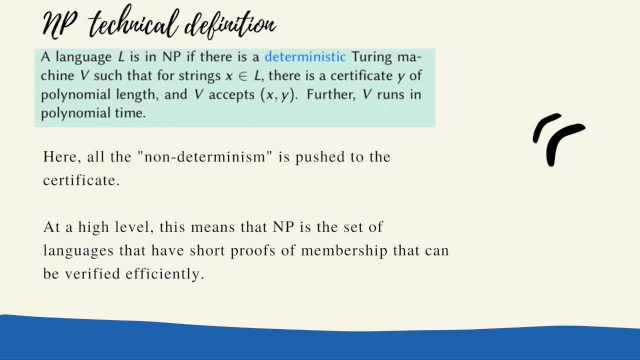 And know that it's completely okay if you do not understand this definition, but this is a definition that is actually thrown in a lot of graduate and undergraduate computational complexity courses And this is a definition that defines NP using a deterministic Turing machine. Know that we actually defined it using a non-deterministic Turing machine. 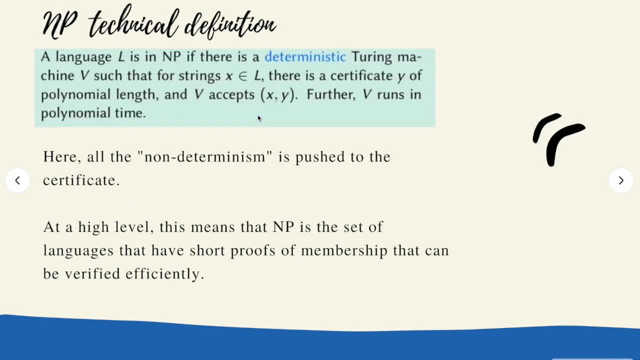 That was definition one. Definition two takes a deterministic Turing machine, let's call it V, and it takes in all instances of all strings in the language and it's an NP. If there is a certificate Y of polynomial length, the certificate is of polynomial size and V accepts Rx, which is the problem, or an instance of the problem. 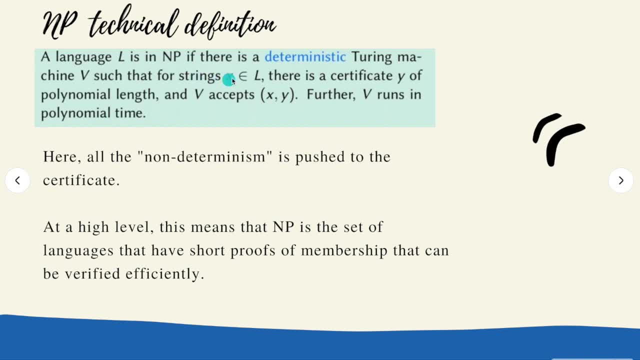 An instance of a string X that is in L, Y, which is the certificate. So it takes in both X and Y and it accepts V, and then it does it in polynomial time. So if a language, L, is said to be an NP, if there is a deterministic Turing machine, V, such that for all strings X that belongs to L, there is a certificate Y, 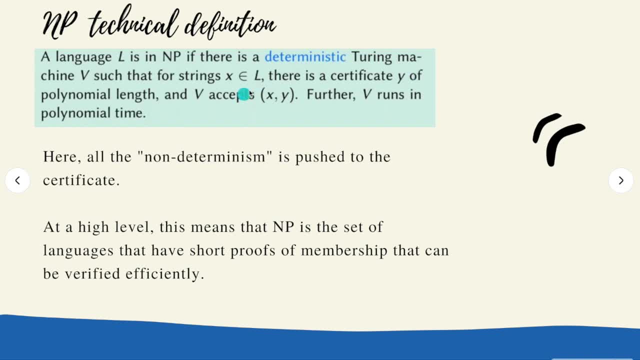 Of polynomial length and V accepts X, Y and it does it in polynomial time. That is the technical definition of NP and slightly not intuitive in the first glance, but it's very useful when you have to prove a lot of things. prove a problem is an NP. 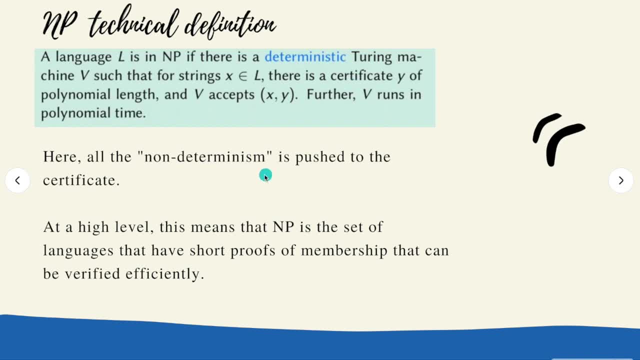 What you basically do is you try to get a certificate and you just use a definition And then prove that the given problem is an NP. Note that all the non-determinism is pushed to the certificate. Like, I mean, I haven't really mentioned how you get the certificate, but essentially all the non-determinism is pushed into the certificate. 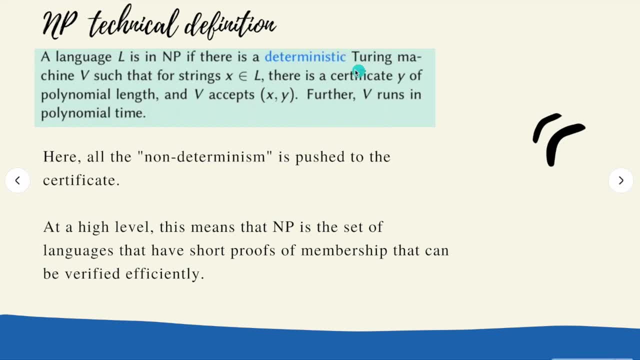 And then you can use a deterministic Turing machine to actually use X and the certificate to actually accept the problem or decide the problem At a very high level. this means that NP is a set of languages that have short proofs of membership. short proofs of membership meaning the certificate is of polynomial length and it's three o'clock. it can be verified efficiently. 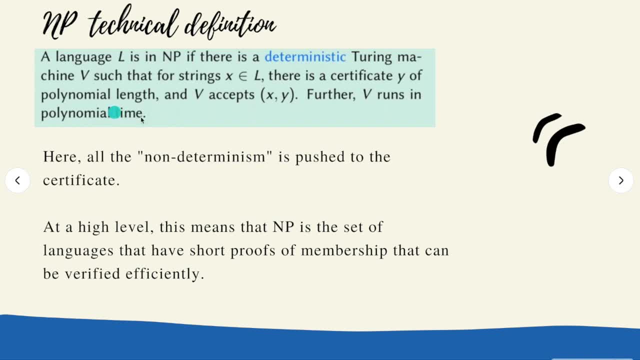 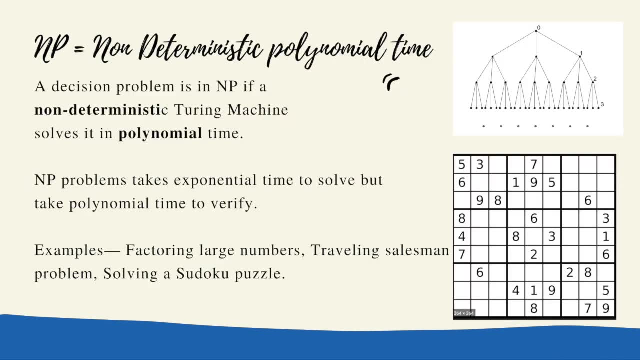 It can be verified efficiently, meaning we have a polynomial time algorithm. So this is the technical definition of NP. It's completely okay if you just understand the previous definition, and this is just for people looking for a slightly more advanced. So for those of you looking for something like ten one and five, a ten hoc plus a mystical definition, 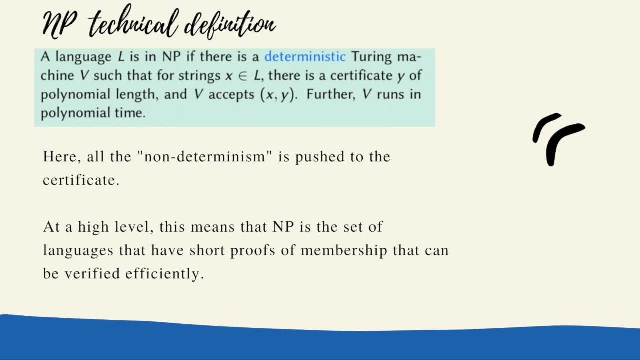 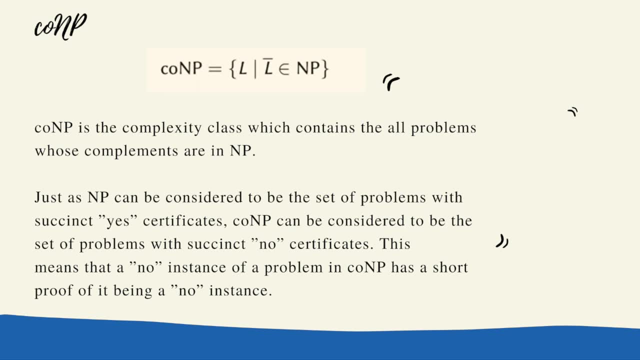 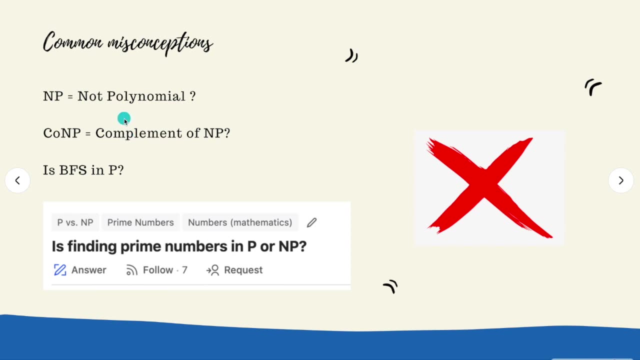 It is an Nそうだ and ST is a definition that is used in uh your undergrad and uh graduate level courses. Um, let's define something called coin ping. again, It's very comment to actually uh how a misconception. 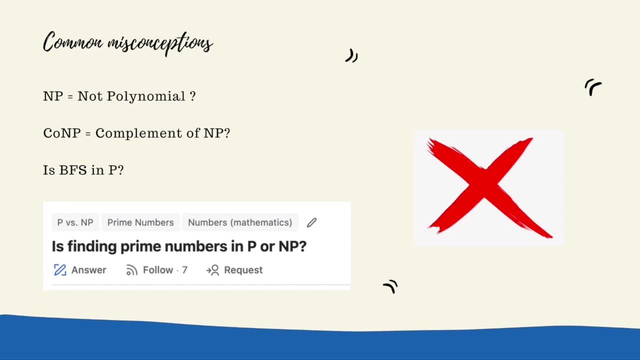 Uh, in fact, like, let me go through the misconceptions once, uh before, actually like uh, lawsuit efendimis goal stand for not polynomial, it is non-deterministic polynomial, and co-np is not the complement of np. 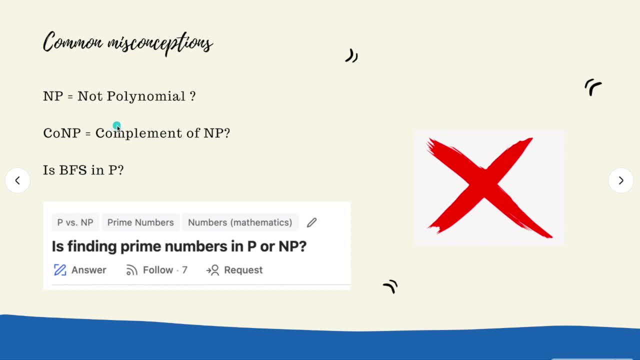 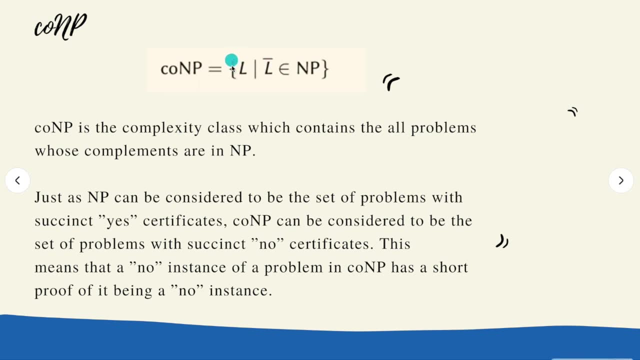 again a misconception. uh, it's. uh. in fact, co-np is a complexity class which contains all problems whose complements are in np. like a language l is said to be in co-np, in the class co-np if l complement, if the complement of the language like belongs to np. 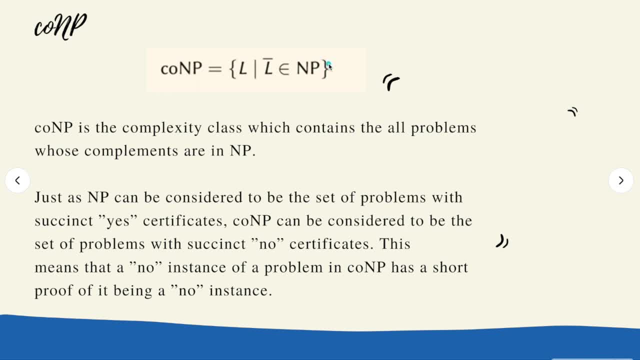 for example, like the problem finding prime is in co-np, because because the complement of that language. the problem is basically to find, to prove that x is not in prime. and to prove that x is not in prime we have to prove that x is in composite and x is a composite number. and that is again an np problem, because to prove 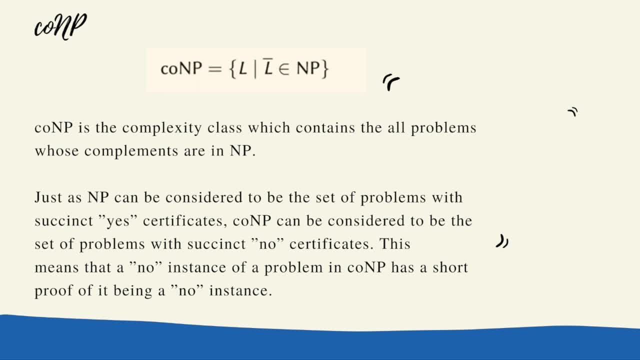 something is a composite number, we have to prove that it's not prime, and that is an np. so this problem is an np and hence that is the definition of co-np. co-np is a complexity class which contains all problems whose complements are in np. 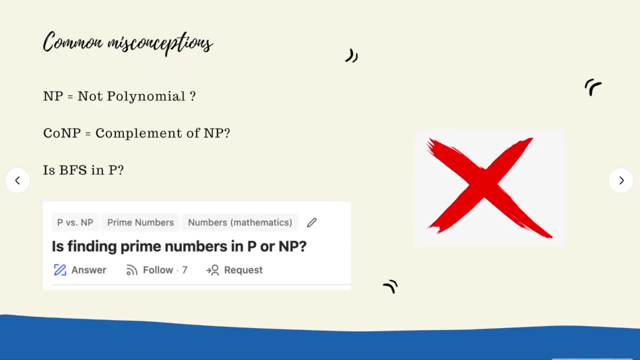 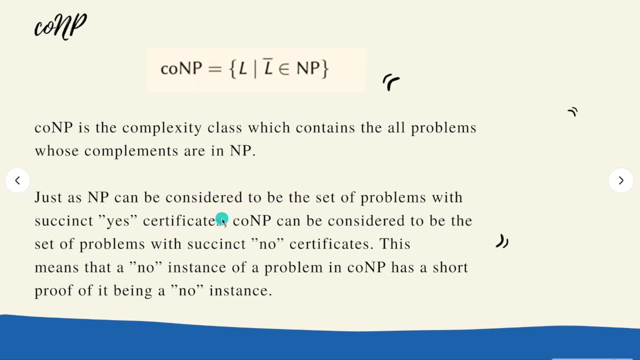 it is not again the complement of np. uh, just as np considered is considered to be the set of all problems that succinct, yes certificates, co-np can be considered to be the set of all problems that succinct very clear: no certificates. this means that a no instance of a problem in co-np has a 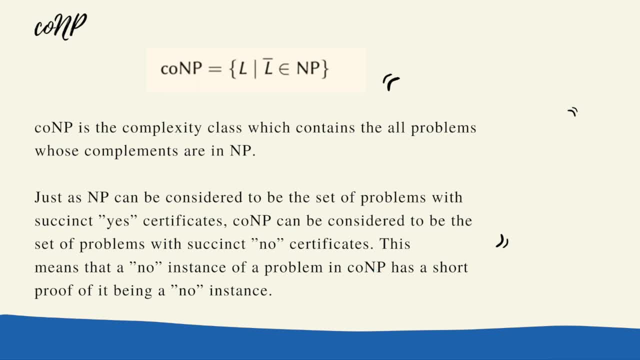 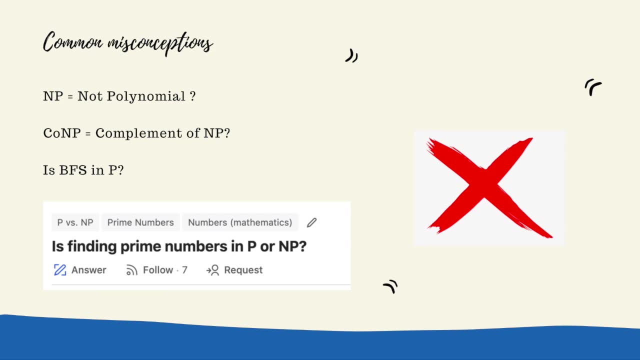 short proof of it being a non, uh, no instance. uh, this is exactly the definition we use for np, except for this is uh. in this time we use it for a no, no certificate or no instance. the uh, the third misconception, or very commonly uh uses like. people ask like if, if an algorithm? 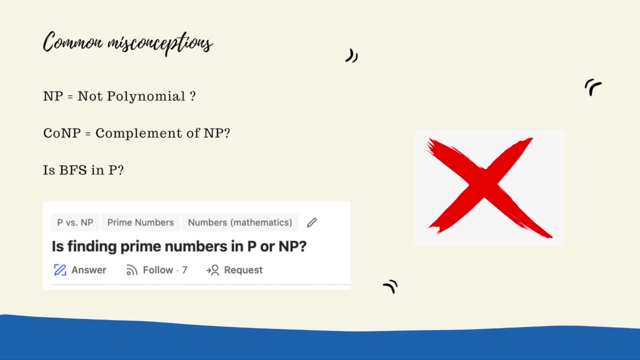 that they've written is in p or np. that again doesn't make sense because, uh, the computation complexity classes are defined for decision problems. and note that an algorithm is not a decision problem. an algorithm is just a way to solve the problem and uh, it's like it is meaningless to ask things like: is bfs in p or np? i mean, 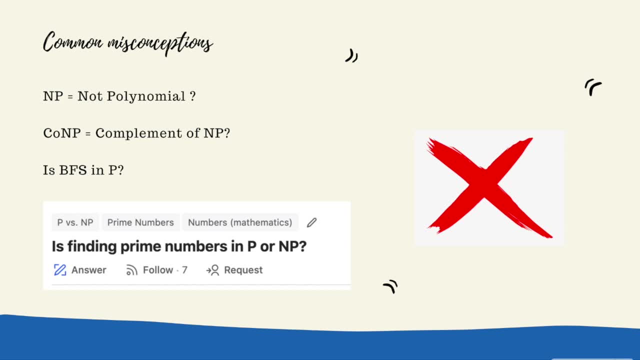 like it does not have a meaning. and again, this is a question that i found in cora and it's uh, it's asking if it's finding prime numbers in p or np. again, this is not right. this is ambiguous, because one like finding prime numbers is not right. there's got to be some sort of solution here. 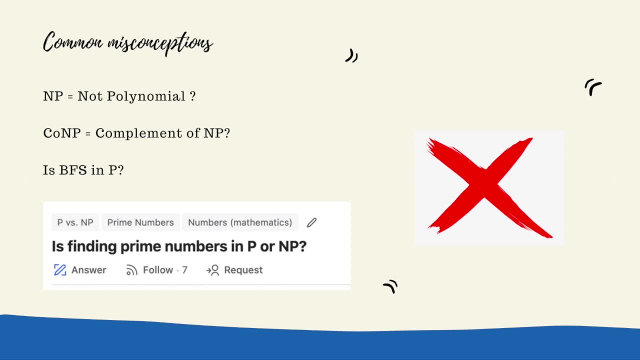 not a decision problem, like asking that if x is prime, that is a valid problem, to ask a valid decision problem, and that can be, like you know, like found off to be in p or np, but again you note that if a problem is in p, it's also in np. in other words, p is contained in np. so if someone 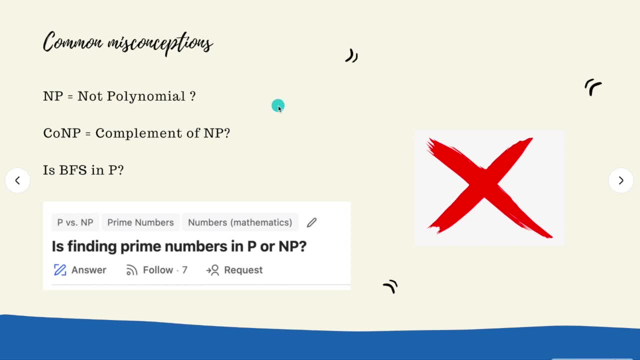 proves a problem is in p, it also implies that a problem is in np. so this question is incorrect, because you're asking finding prime numbers, and that is not a decision problem, and you're asking a question that is not a decision problem and that is not a decision problem and that is not a. 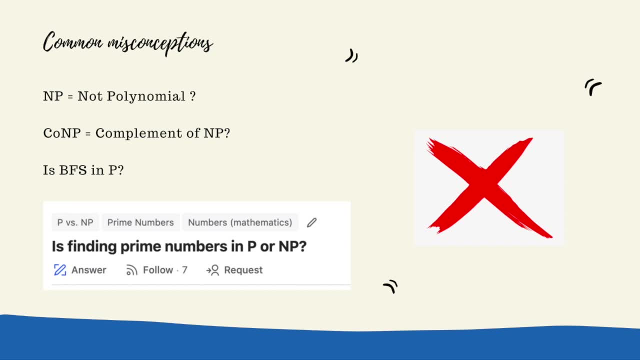 if p or np. that means you are trying to ask if, like, they are mutually exclusive classes and they are not- p is in fact contained in np. we do not know if p equals np. that is a. that's a puzzle. that's actually something people are trying to solve. it's a mystery. 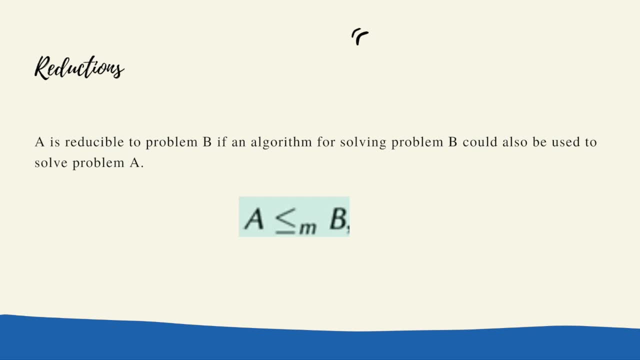 but most rational people believe p is not equal to np, but that's a story for another day. and yes, let's go or let's define what reductions are. a is reducible to problem b if an algorithm for solving b can also be used to solve problem a, that is, if i can solve b. 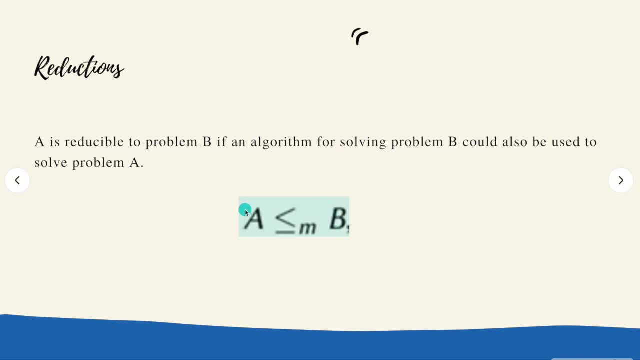 that also means i can solve a, because the yes instances of a can be mapped to all s instances of b and the no instances of a map to no instances of b. so the yes maps to yes and no maps to no, and i'm trying to get an yes or no for a. so if i can go from a to b in polynomial time, note that it's a polynomial. 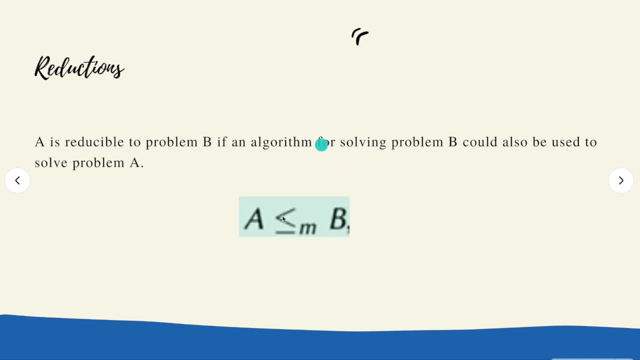 time reduction and i haven't mentioned that, but it's a. reductions are of many kind, but usually the ones we define in computational complexity. there's a bound on the reduction, and you like what to define things like np, complete, to use a polynomial time reduction and, uh, to go from a to b. 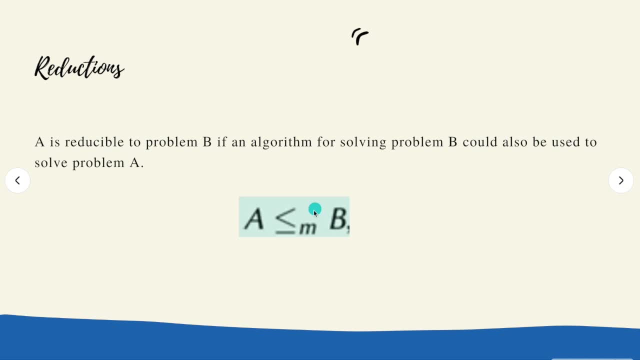 uh, like, if we can solve b, there's an algorithm to solve b. that also means we can solve a, because yes of a maps, yes of b. so if we can get a- uh- an answer from b, we already have an answer for a. so that is reduction from a high level. 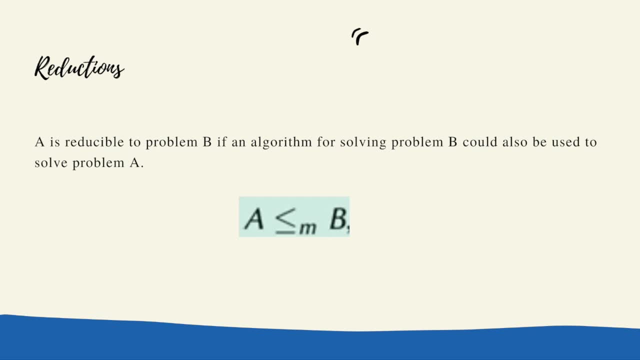 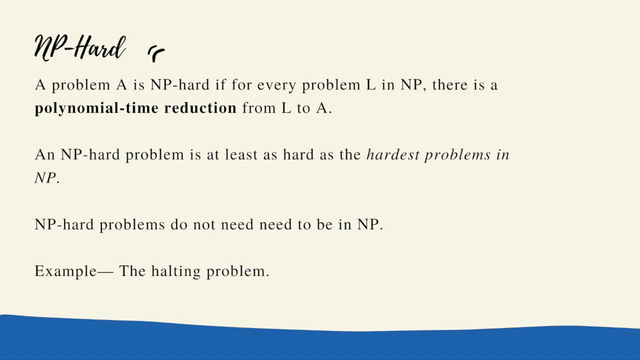 it's a much more complicated topic and i wouldn't be covering this in depth in this video. okay, let's try to define np-hard with the definition of reduction, since we know what a reduction is. a problem a is np-hard for every problem. l in np if there is a polynomial time reduction from l to a. yeah, if a is np-hard. 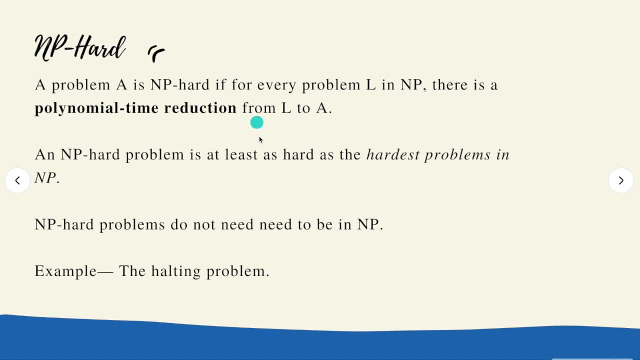 that means like we can reduce every problem in L N P, every problem L in N P, to that problem A which is N? P hard. so the in polynomial time. so that is what this means. this will become much more clear with the help of a visualization. that means an N P hard problem is at least as hard as 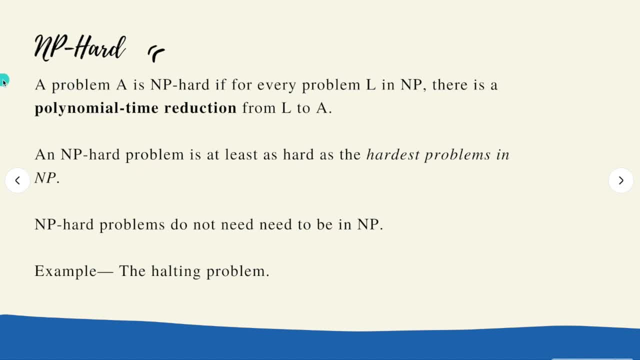 the hardest problems in N P, like, let's say, they have. there are so many problems in N P and this N P hard problem which need not be in N P, which need not be N P, and this problem is at least as 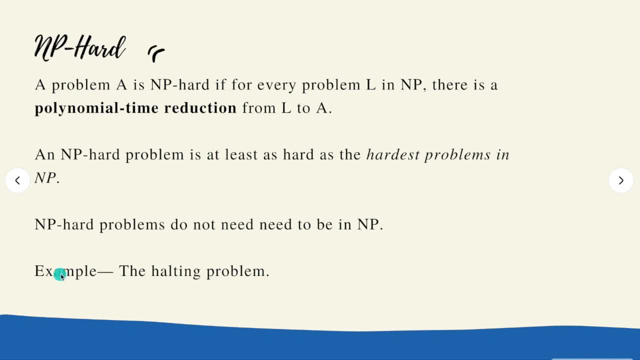 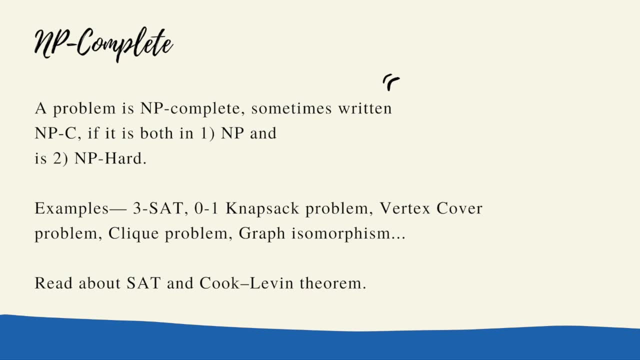 hard as the hardest problems in N P. an example of an N P hard problem would be the halting problem. yeah, let's define N P complete and then let's take a look at a diagram to make the definitions clear. and a problem is said to be N P complete if it satisfies two conditions and it's written. 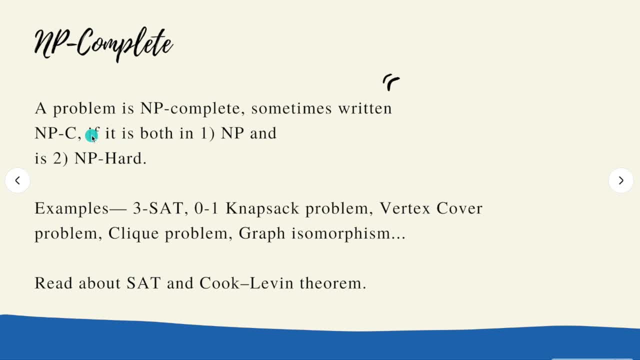 as N P C sometimes, but that's a notation for N P complete and a problem. is N P complete if it can be both in, if it satisfies the following two conditions: if it is an N P, that is a one, and it's N P hard. so an N P complete problem is just an N P hard problem, that is. 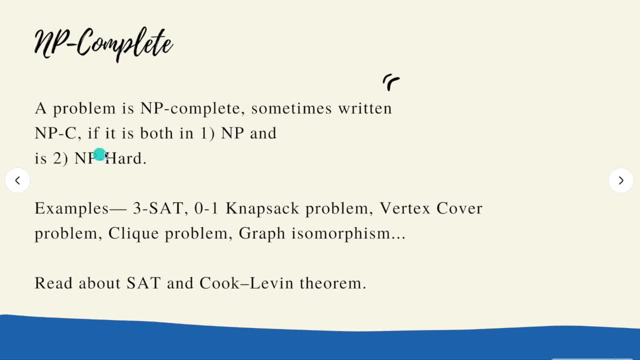 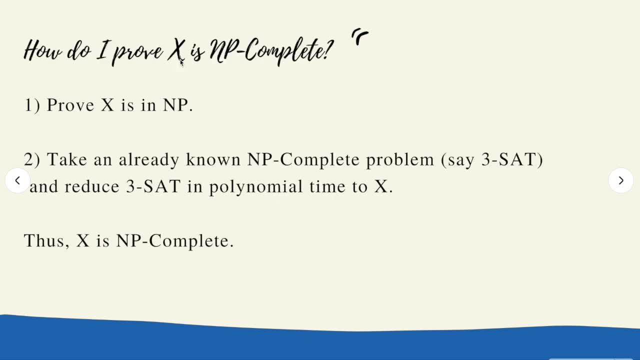 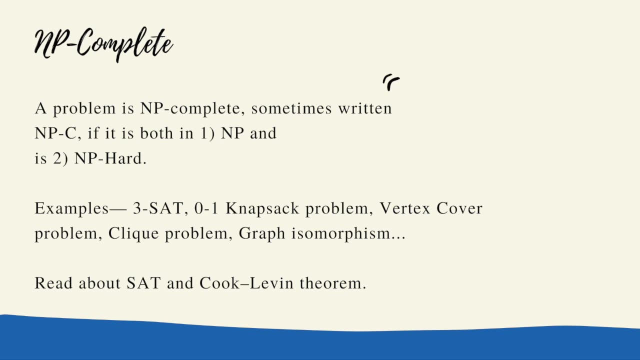 always also an N P and hence like to show that a problem is N P complete. what do we do? we actually like to show that a problem is N P complete. we actually just like need to prove that one it's an N P and two, all problems, like all problems in N P, it reduces in polynomial time. two. 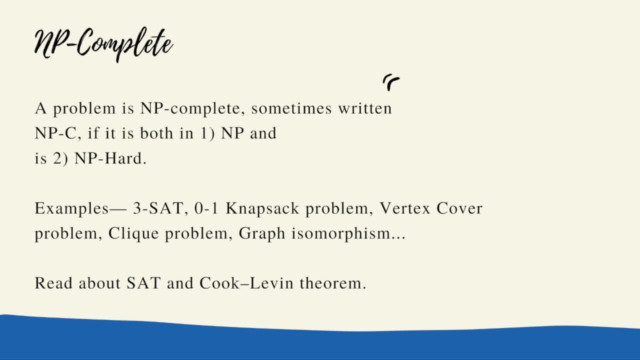 problem, like the problem we are trying to prove, that that is an N P complete, and examples of N P complete would be three SAT. I would advise you to read about what a SAT problem is. in fact, three SAT is just a Boolean satisfiability problem where it's more restrictive that every 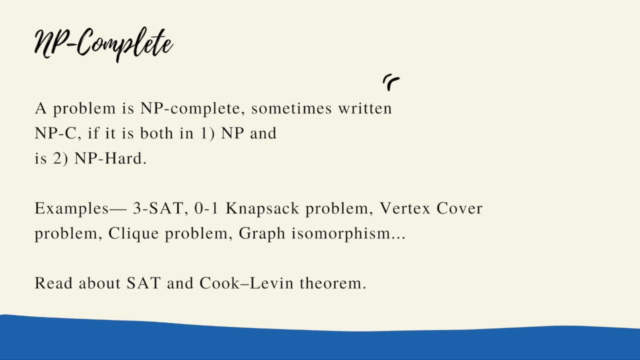 class can only have three literals, so hence three SAT. and we have the zero knapsack problem, we have the vertex curve problem, we have clique, we have graph isomorphism. they're all N? P, complete problems. and please read about SAT and cook-levin theorem. cook-levin theorem, in a nutshell, is: 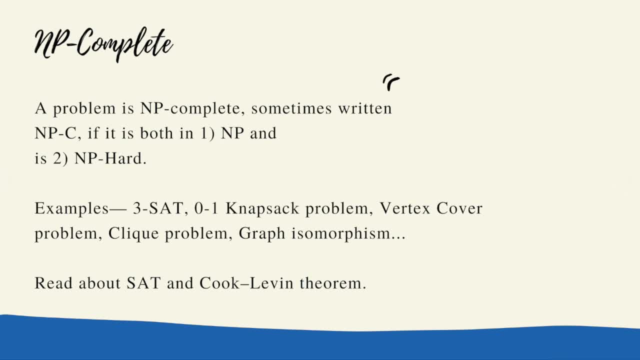 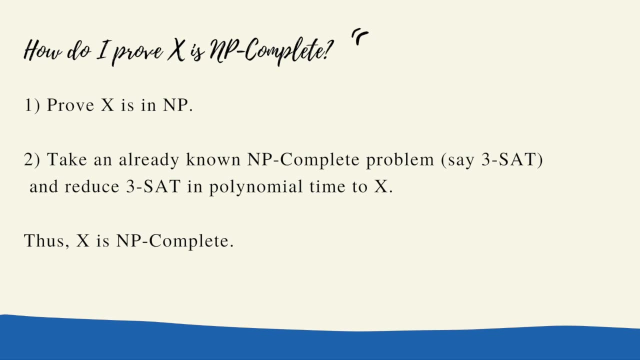 just like the first N P complete problem that is proven, and that was satisfiability problem, the SAT problem. hence we know that three SAT is N? P complete. and why is this useful, you may ask? this is useful precisely for this reason: to prove that a new problem, X, is N P complete. so how do you do this? first you need to prove. 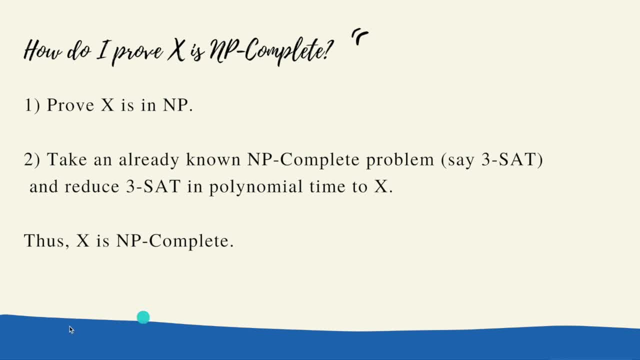 that X is an N P. and second, you need to prove: take an already known N P complete problem. this is the result of cook-levin theorem and we reduce that three SAT problem in polynomial time to X, to this problem. we are trying to prove that is N P complete and thus X is. 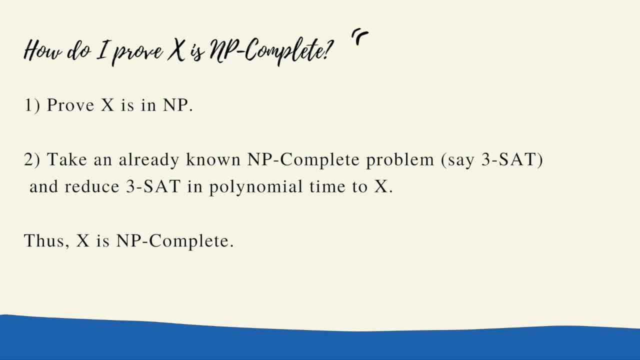 N P complete. note that it need not be three SAT. it can be any known N P complete problem that we've already proved to be N P complete. we can you proven to be N P complete. we can use that result to actually reduce in polynomial time from that known N P complete problem. 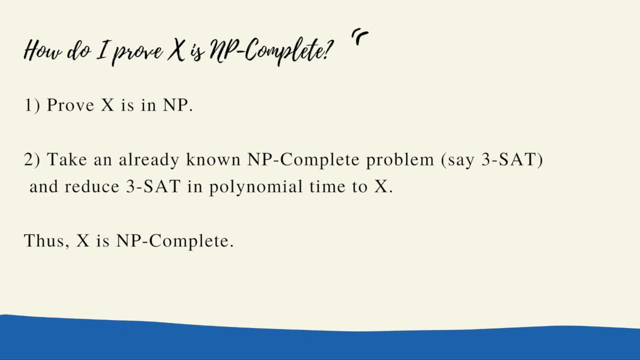 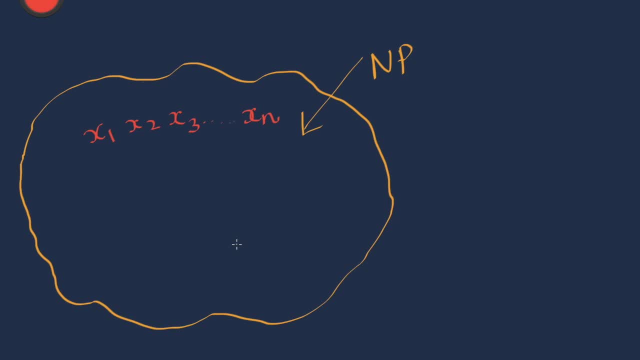 to our problem and then we can prove that X is N P complete. okay, how do we prove that a problem, A, is N? P complete? we can prove that A is N P complete by picking any problem that is already proven to be N. 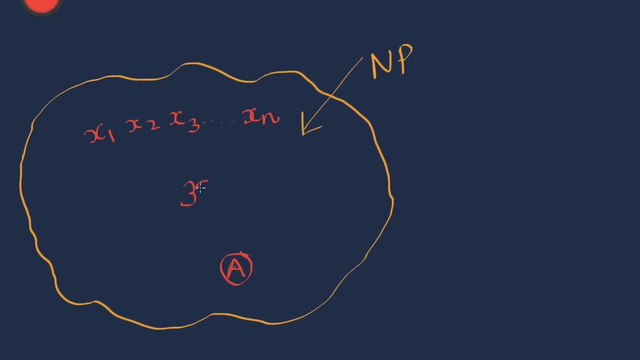 P complete, and because to show something is N? P complete, we need to prove that every language that is an N P- X1, X2, X3 and so on up to X in- is an N? P, and that reduces to our problem in polynomial time. 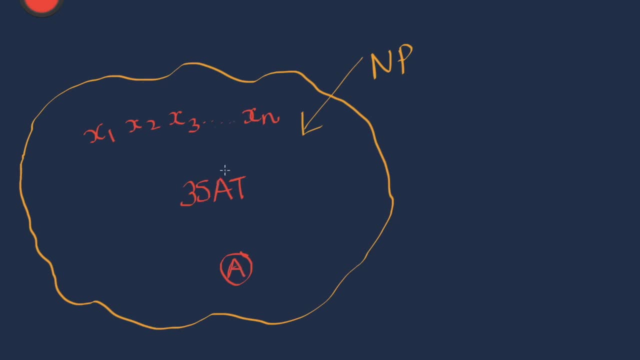 and that can be pretty hard to do. Instead, we already take a known NP-complete problem. This is the result of Cook-Levin theorem, and someone already did the work for us. Hey, why not use that? So this makes it much simpler, because, since we already know that, 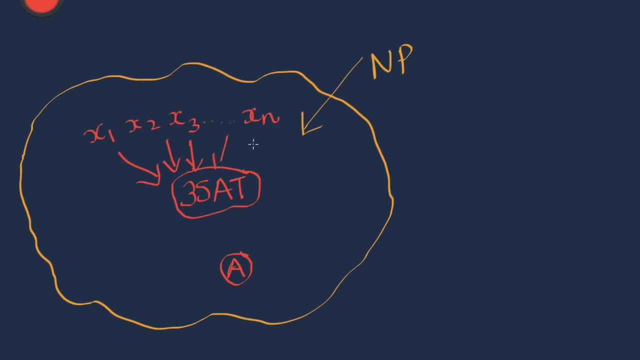 3SAT is NP-complete. that means every problem in NP can be reduced in polynomial time to 3SAT. And if we can show that 3SAT can be reduced in polynomial time to A, to our problem A, that's the only chunk of work we need to do And this also implies that every problem. 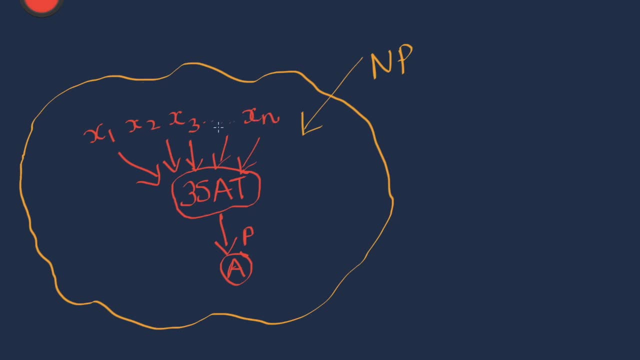 x1,, x2,, x3, and xn, which is in NP, is actually reduced in polynomial time to our problem, A, and that is the definition of NP complete. So that's the definition of NP complete, because A is in NP. that's condition 1. 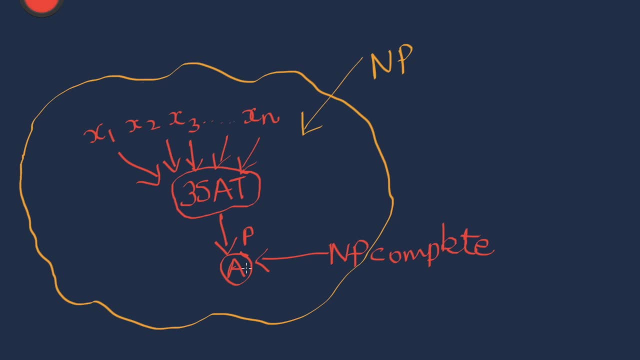 and condition 2 was that every problem x1, x2, x3 and so on up to xn, every problem that's in NP, is also reducible in polynomial time to our problem A, and hence A is NP complete. So this is how we prove a language A or a problem A is NP complete, by actually picking any problem that's already. 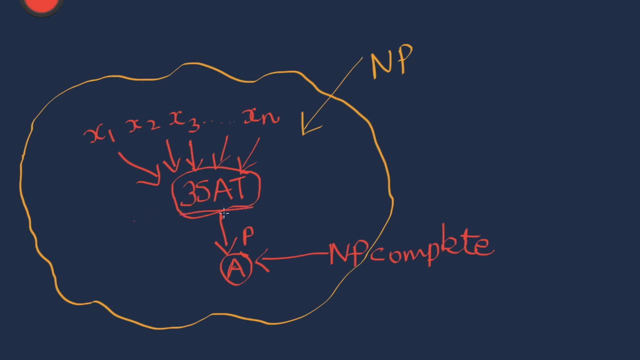 NP complete and in our case we picked a 3SAT and we just proved that 3SAT reduces to A in polynomial time and once we do that, you can see that the problem A is NP complete. Our proof is done and we can show that A is NP complete. 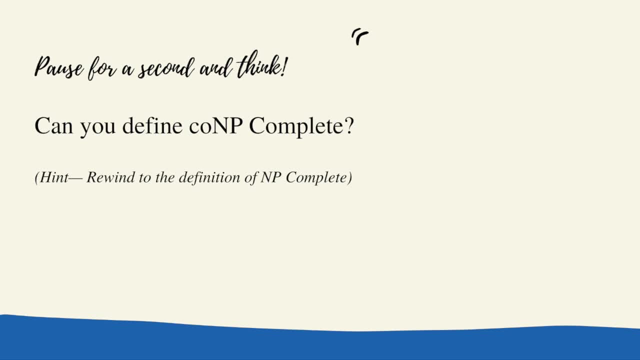 Okay, I want you to pause for a second and think if we can actually define something like what is co-NP complete? We talked about co-NP, we talked about NP complete, and can you pause for a second and think what can be the definition of co-NP complete? This is because it's often like 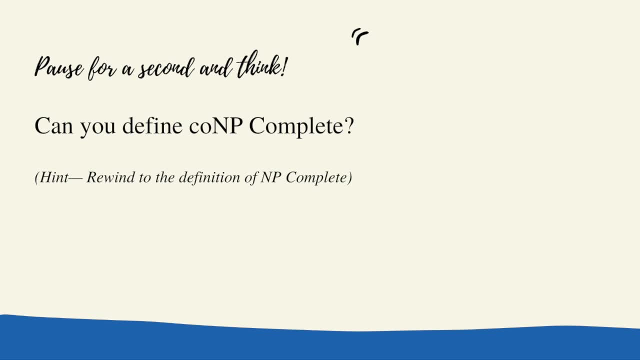 very common to define things like C-hard, C-complete, etc. where C is a computational complexity class, like people talk about what is P-complete, what is like for a lot of classes like, for example, what is NL-complete? So many extensions are the same and they follow the exact same template, like 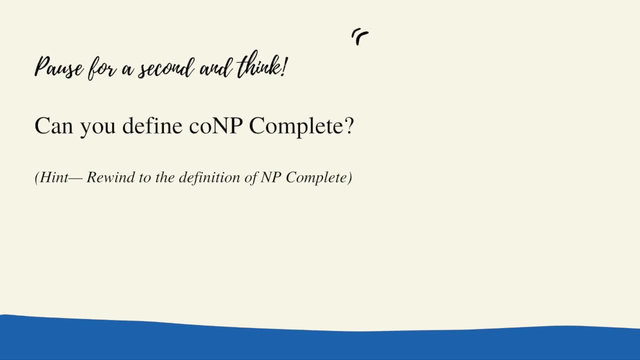 I mean like one. you have to prove that for a language should be C-hard. you just need to prove For language to be C-complete, you need to prove it's in C and it's also C-hard. basically, to prove that it's in C-hard, you have to prove that it's one in C and 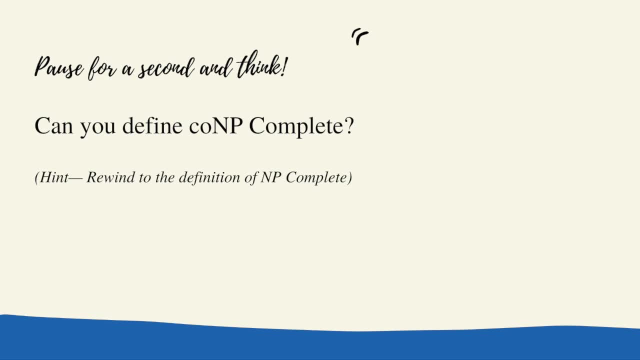 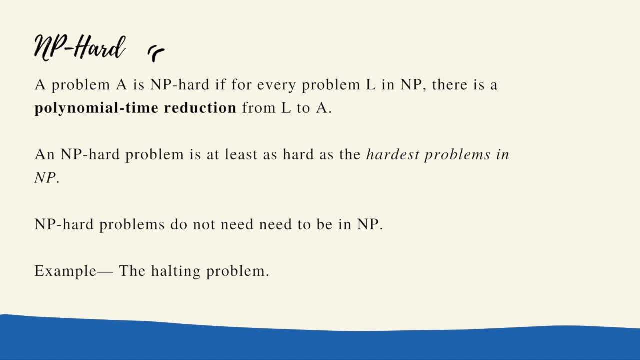 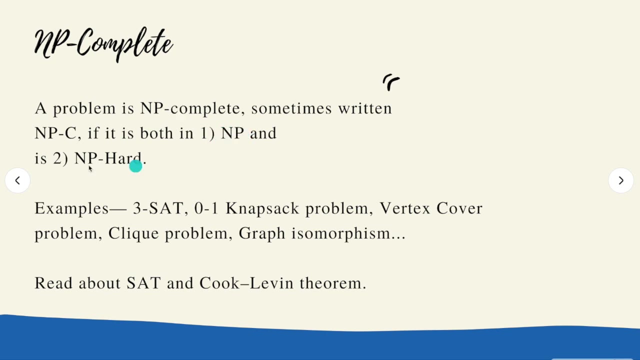 two, you have to prove it's C-hard. An example was just what we discussed. and yeah, to prove that it's C-complete, you just need to prove that it's in C. and two, it's C hard. In this case, C is NP. the class we are referring to is NP. 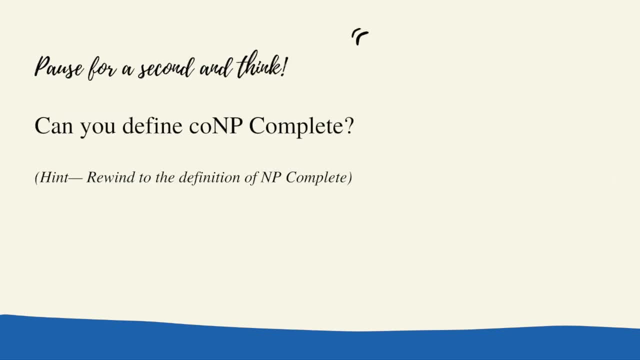 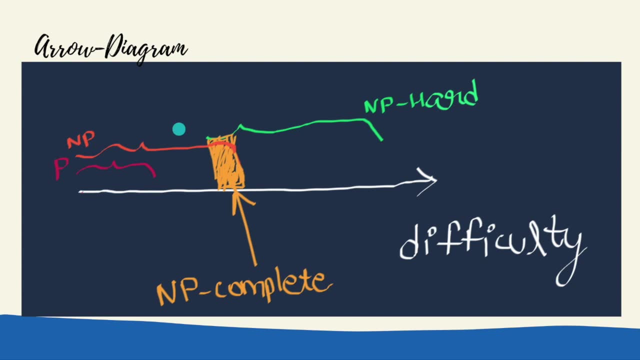 So just pause for a second and try to define what co-NP complete is. Yeah, This is the diagram. We have P and I told you that P is contained in NP And we have the NP hard class And if you have a line of difficulty, 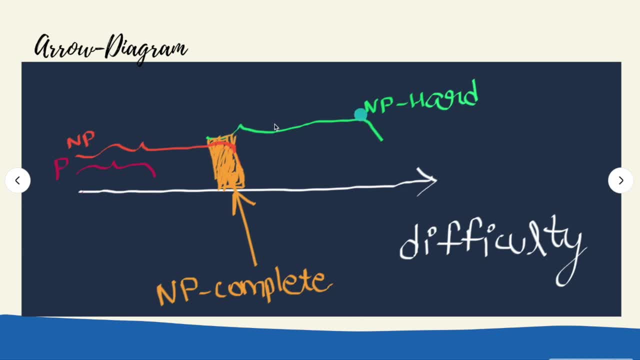 this is what it would look like. And we have the NP hard class And I already told you that all NP hard problems need not be in NP. So- and this the part where it overlaps- it need not be just a point. 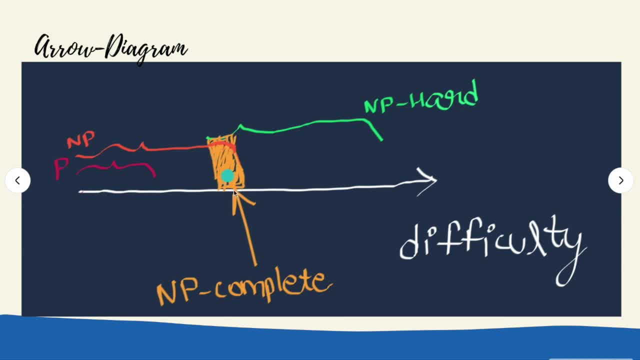 The part at which it overlaps is the class NP complete, Because this class is an NP and it's also NP hard. So by definition, this is NP and NP hard. So that's making it NP complete. So I hope this is clear. 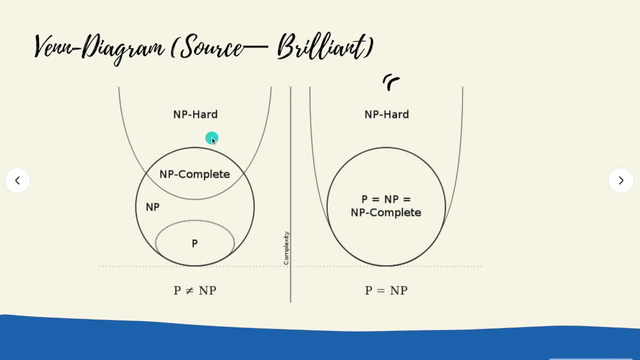 It'll become much more clearer. It'll become clearer after this Venn diagram, I'm assuming P is not equal to NP in the left hand. So we have P which is contained in NP- Yeah, which is contained in NP- And we have NP hard, which is actually not entirely in NP. 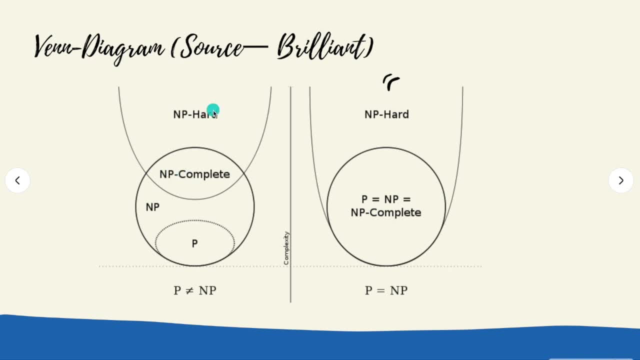 like I already told you, And that's the overlap between NP hard and NP, is NP complete? And if P- if someone in the future it could be you- If someone from future actually proves that P equal to NP, which is unlikely. but if that happens, 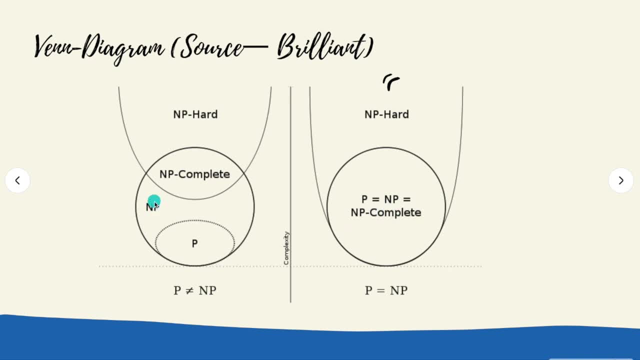 then this NP collapses to P, because NP equal to NP. that would mean, like you know, the whole thing collapses And thus we have P equal to NP, equal to NP, complete, And the whole Venn diagram would become a lot more easier. 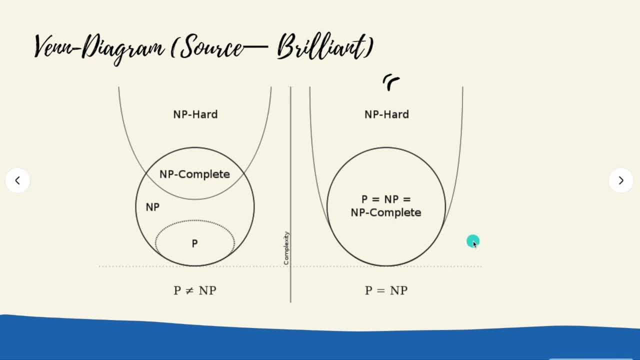 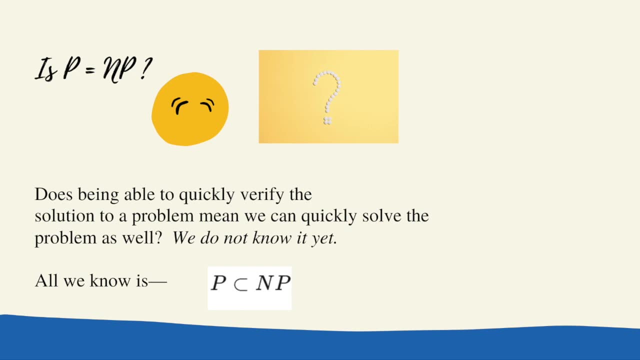 If someone proves that P is equal to NP, So that is the result we have on the right hand side. Yeah, and that is the problem of P equal to NP, P versus NP, And that is like what it means. It's one of the most millennial price problems. 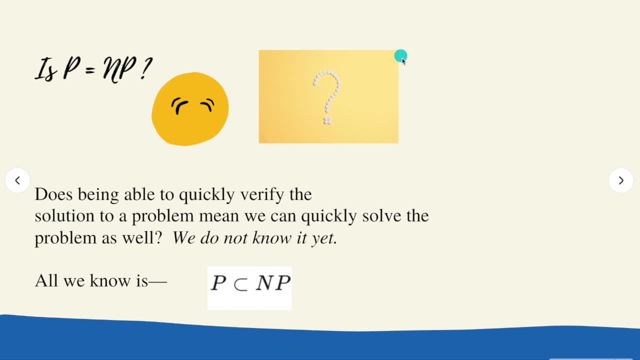 It's by The Clay Institute And it's a graduate school, So it's one of the most millennial millennial price problems. it's by The Clay Institute And it's one of the most millennial millennial price problems. it's the millennium price problems, millennium price problems, and it actually 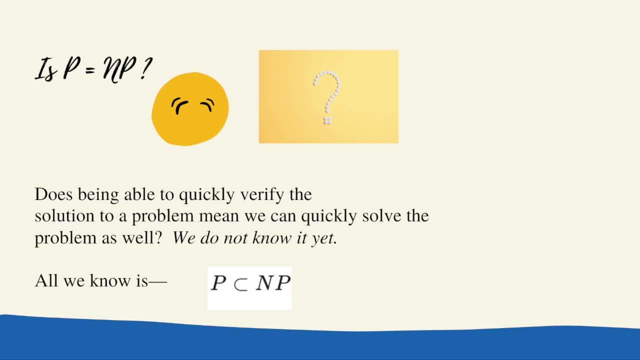 can be described simply as this: Does being able to quickly verify the solution to a problem mean that we can also quickly solve the problem? I mean, does it like if we can verify a solution to a problem, does it quickly that mean, does it also imply that we can solve the problem? 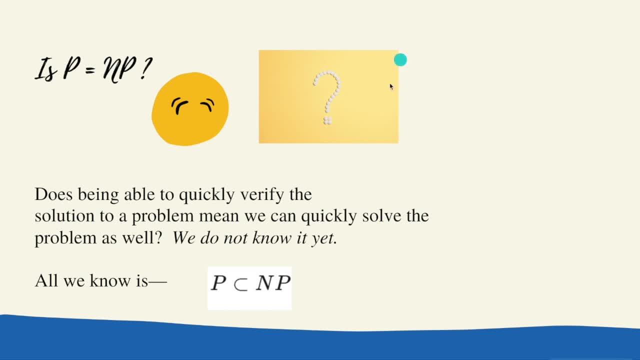 So that is the question of P versus NP in a nutshell. We do not know that yet And all we know is that, for now, is that P is contained in NP. So if P equal to NP, the whole thing collapses and we'll have just a circle of sorts and where NP collapses to P. 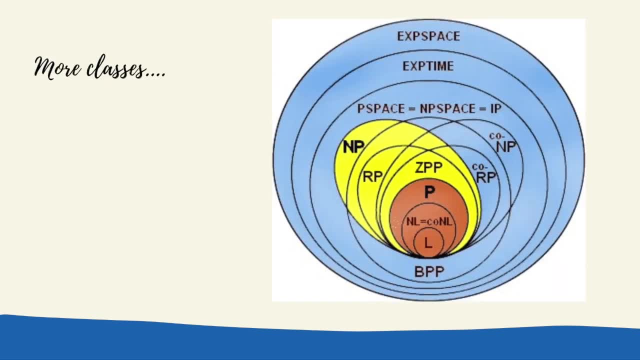 There are a lot more classes than what I have just described, but that captures the basic fundamental classes that are introduced to you in algorithm scores. Of course there's the randomized complexity class, There's P, there's NP, I mean, there's RP, there's co-RP, there's ZPP. 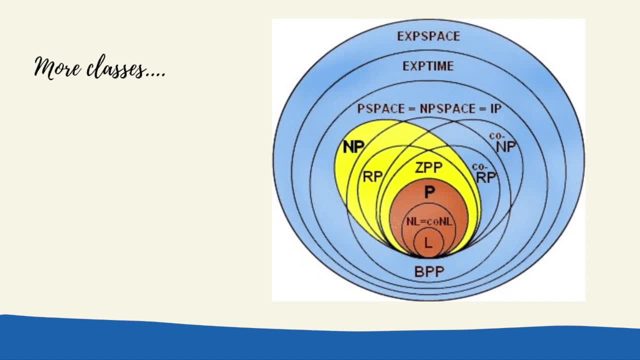 there's BPP, there's L, which is the space complexity classes, L, NL, co-NL, and you have a lot more classes like sigma 2, pi 2, and so on, And maybe you can discuss that sometime. 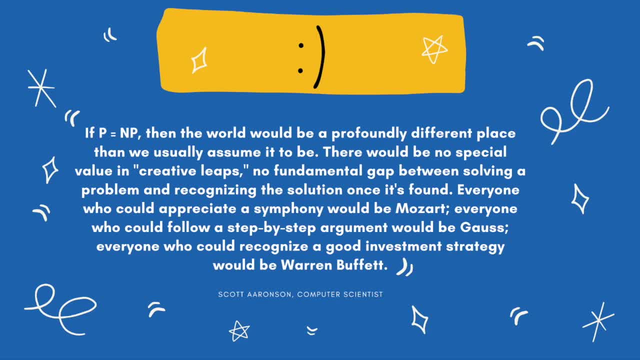 In the future. This is a very- this is a very fascinating quote I came across. If P equal to NP, people actually like talk about things like protein folding algorithms can be solved, and quickly, And if those can be solved quickly, we'd have the cure to cancer, or you know all these. 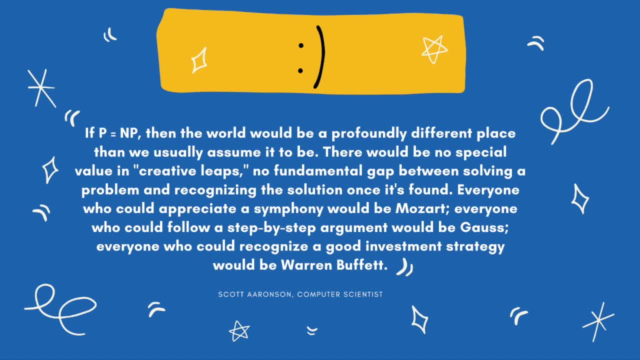 net banking systems. internet banking systems would, it would be prone to hacking, So we'd have to do a lot of hacking because, basically, cryptographic algorithms would be easier to crack. So those are very interesting examples, but this quote I found it more succinct and I 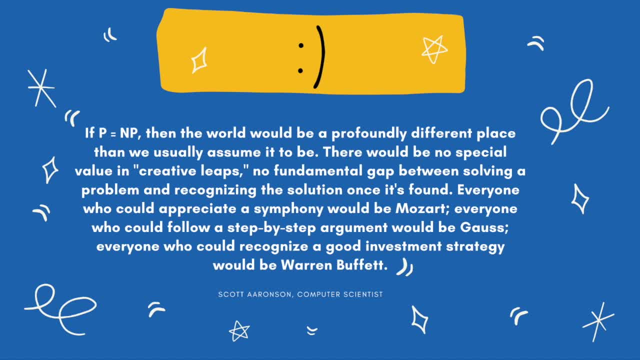 found it very interesting, And it's this. it's a quote by Scott Aronson, who's a very popular computer scientist, And he quotes: if P equal to NP, then the world would be a profoundly different place than usually assumed it to be. There will be no special. 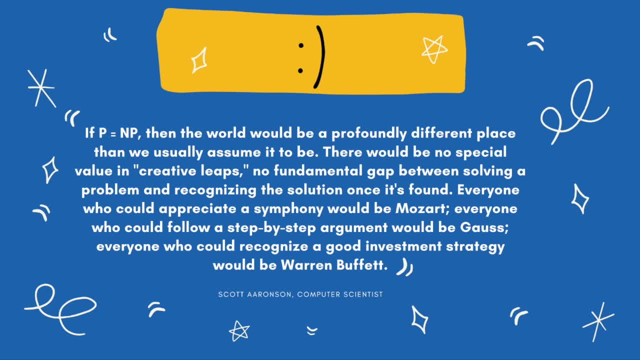 value in creative leaps. No fundamental gap between solving a problem and recognizing the solution once it's formed. Everyone who could appreciate a symphony would be Mozart. Everyone who could follow a step by step argument would be Gauss. Everyone who could recognize a good investment strategy. 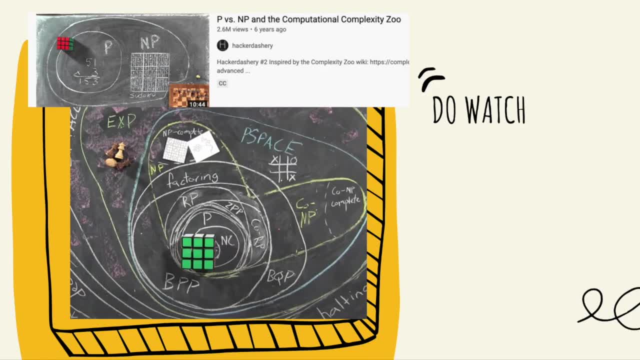 would be Warren Buffett. With that I conclude, and I would highly recommend you to watch this video. It has beautiful animations and it captures the idea very well. Thank you for watching. I'll see you in the next video. Bye, Bye. 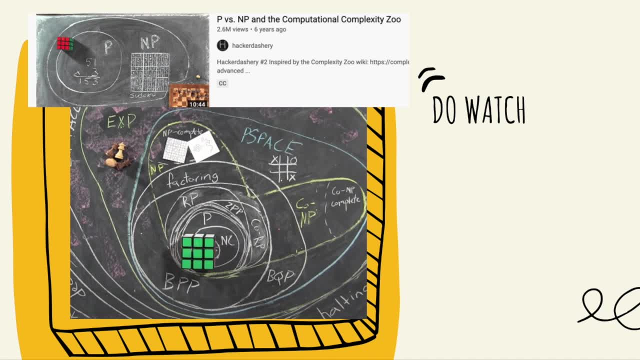